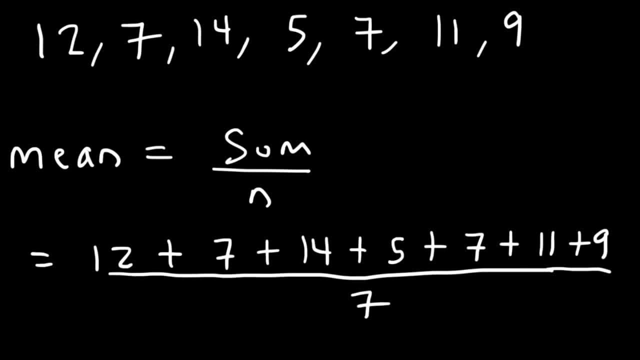 And since there are seven numbers, let's divide it by 7.. So the sum of the seven numbers is 65.. 65 divided by 7 is equal to 9.285, or 286 if you round it. So that's the arithmetic mean of those numbers. 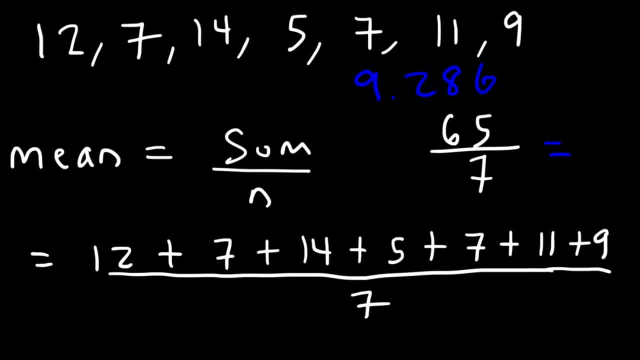 Now, what about the median? How can we calculate the median of this data set? What do you think we need to do in order to find it? To find the median, it's going to help if you arrange the numbers in increasing order. The lowest number is 5, and then we have two 7s. 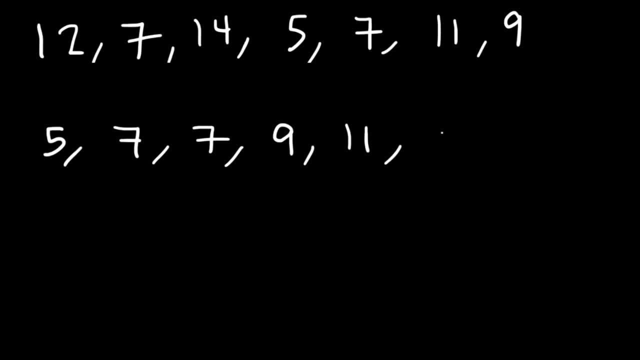 Next, we have a 9,, 11,, 12, and 14.. Now, in order to find the median, we need to find the middle number. The best way to find the middle number is to eliminate the first and the last number. 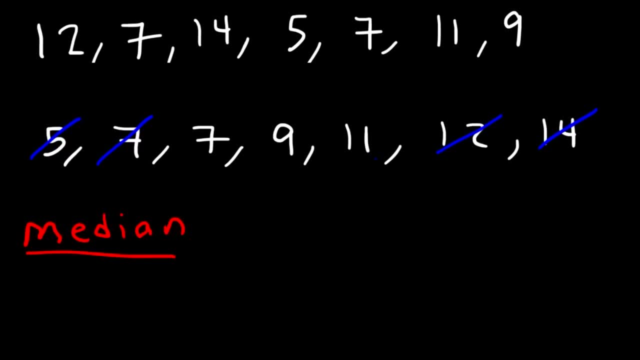 Next eliminate the second number and the second to last number And then eliminate the third and the second or the third one from the left. The one in the middle is the median. So in this example the median is equal to 9.. 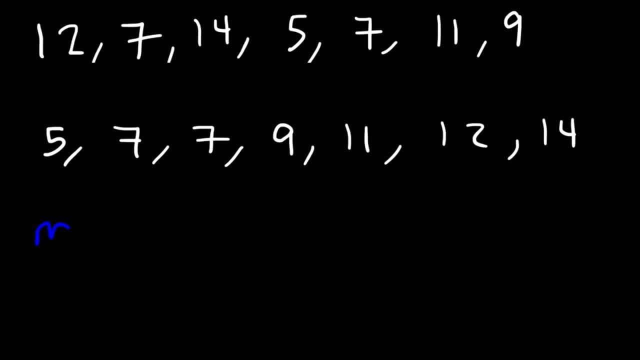 Now, what about the mode? How can we calculate the mode? The mode is simply the number that appears the most often or the number with the highest frequency. Every number appears once except 7.. 7 appears twice, So the mode is equal to 7.. 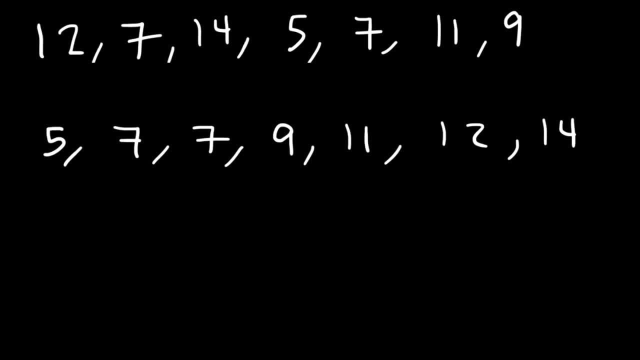 Now, the last thing that we need to calculate is the range. So how can we find the range of this data set? The range is simply the difference between the highest number and the lowest number. The highest number is 14,, the lowest number is 5.. 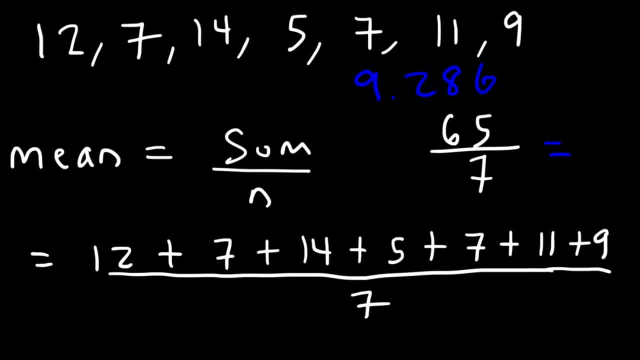 Now, what about the median? How can we calculate the median of this data set? What do you think we need to do in order to find it? To find the median, it's going to help if you arrange the numbers in increasing order. The lowest number is 5, and then we have two 7s. 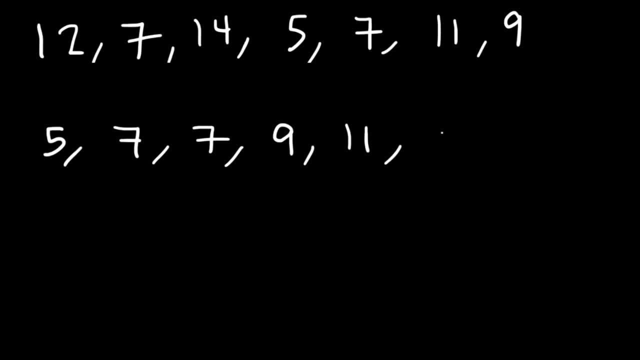 Next, we have a 9,, 11,, 12, and 14.. Now, in order to find the median, we need to find the middle number. The best way to find the middle number is to eliminate the first and the last number. 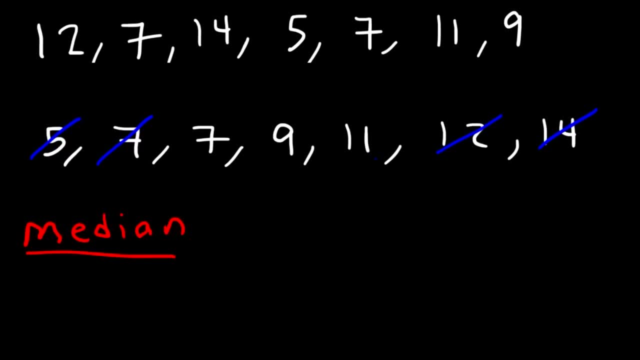 Next eliminate the second number and the second to last number And then eliminate the third and the second or the third one from the left. The one in the middle is the median. So in this example the median is equal to 9.. 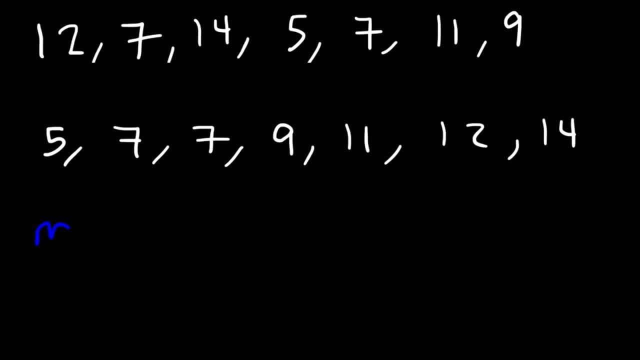 Now, what about the mode? How can we calculate the mode? The mode is simply the number that appears the most often or the number with the highest frequency. Every number appears once except 7.. 7 appears twice, So the mode is equal to 7.. 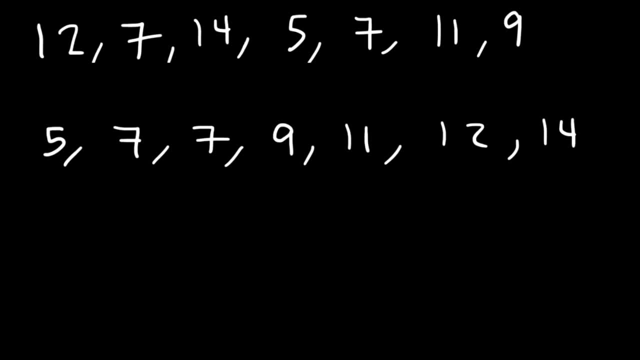 Now, the last thing that we need to calculate is the range. So how can we find the range of this data set? The range is simply the difference between the highest number and the lowest number. The highest number is 14,, the lowest number is 5.. 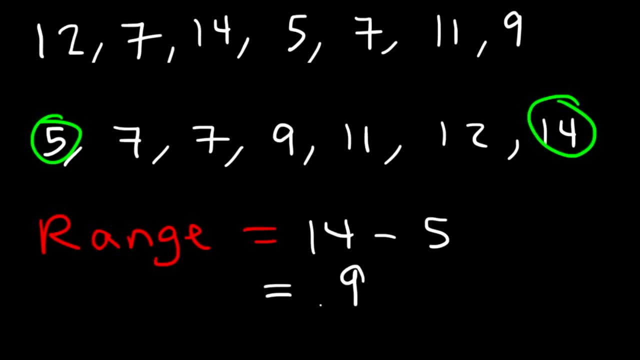 14 minus 5 is 9, and so 9 is equal to the range. Now let's work on another example. So let's say, if we have a data set that contains the numbers 6,, 14,, 8,, 5,, 3,, 11, and 9.. 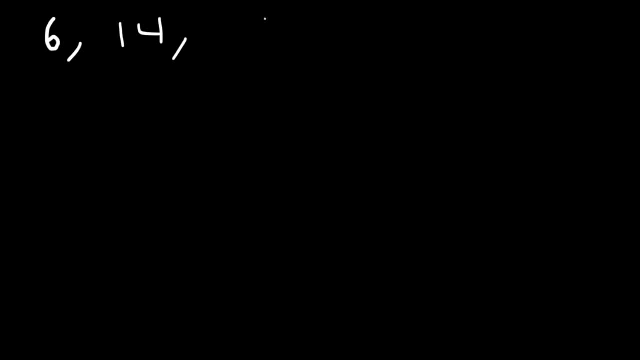 So, if we have a data set that contains the numbers 6,, 14,, 8,, 5,, 3,, 11, and 9.. So, if we have a data set that contains the numbers 6,, 14,, 8,, 5,, 3,, 11, and 9.. 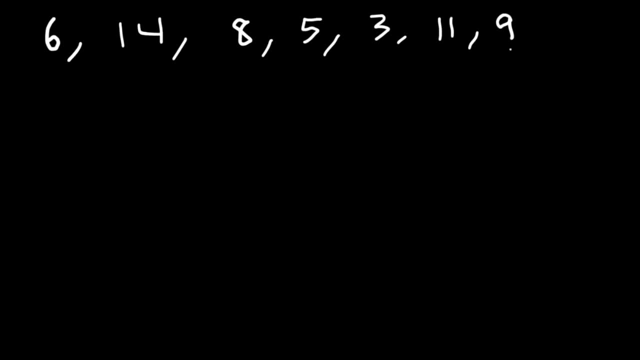 So go ahead, pause the video and try this practice problem: Find the mean, median, mode and range. When you finish, just unpause it and see if you have the right answer. So let's start with the mean, So let's find the sum. 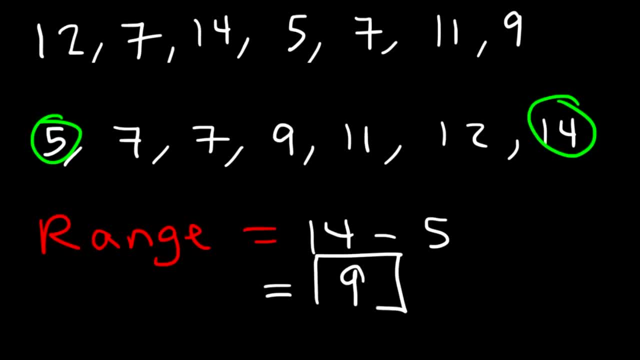 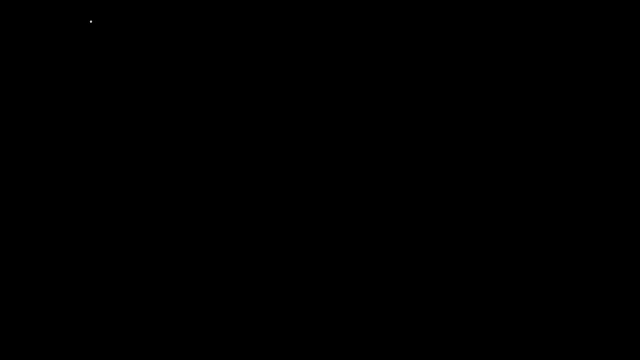 14 minus 5 is 9.. And so 9 is equal to the range. Now let's work on another example. So let's say, if we have a data set that contains the numbers 6,, 14,, 8,, 5,, 3,, 11, and 9.. 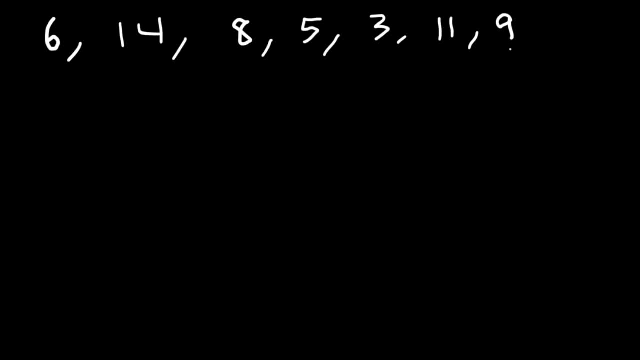 So let's say, if we have a data set that contains the numbers 6,, 14,, 8,, 5,, 3,, 11, and 9.. So go ahead, pause the video and try this practice problem. So let's say, if we have a data set that contains the numbers 6,, 14,, 8,, 4,, 3,, 11, and 9.. 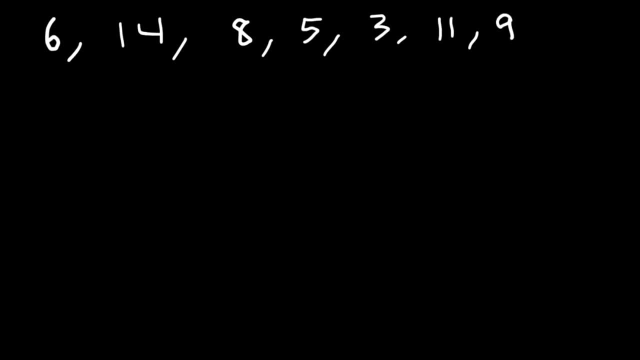 Find the mean median mode and range. And when you finish, just unpause it and see if you have the right answer. So let's start with the mean. So let's start with the mean, So let's find the sum. 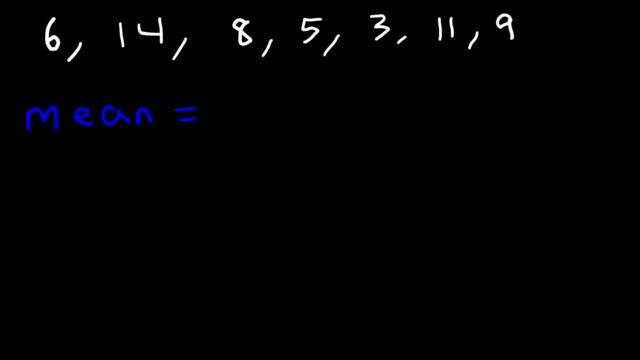 Let's add up the 7 numbers: 6 plus 14 plus 8 plus 5 plus 3 plus 11 plus 6 plus 14 plus 8 plus 5 plus 3 plus 11 plus 7 plus 14 plus 2 plus 3 plus 11. 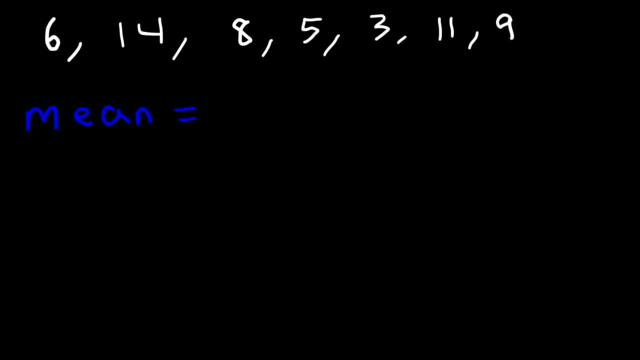 plus 11 plus nine adds up to 56, and there are seven numbers. so we're going to divide it by seven. 56 divided by seven is eight, so the average, or the arithmetic mean, is equal to eight. so now let's go ahead and calculate the median. 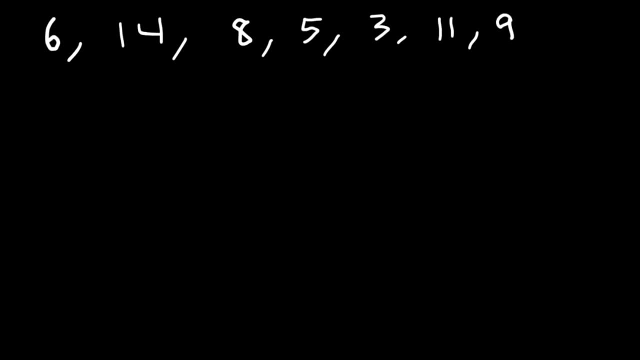 but to do that, let's arrange it and increase in order. the lowest number is three, the next one is five, and then we have six, eight, nine, eleven and fourteen. notice that the middle number is eight. so therefore, the median is equal to the median and the median is equal to the median and the median is equal to. 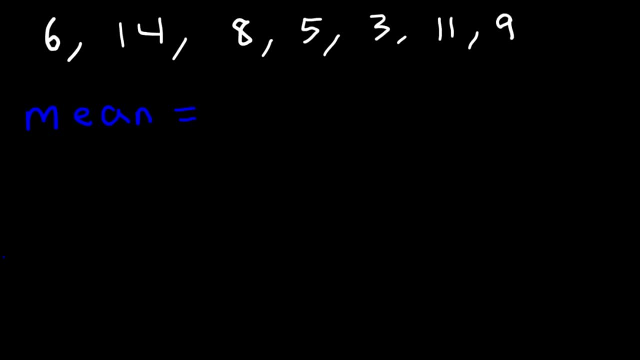 Let's add up the seven numbers: Six plus fourteen plus eight plus five plus three plus eleven plus nine adds up to fifty-six, And there are seven numbers, so we're going to divide it by seven. Fifty-six divided by seven is eight. 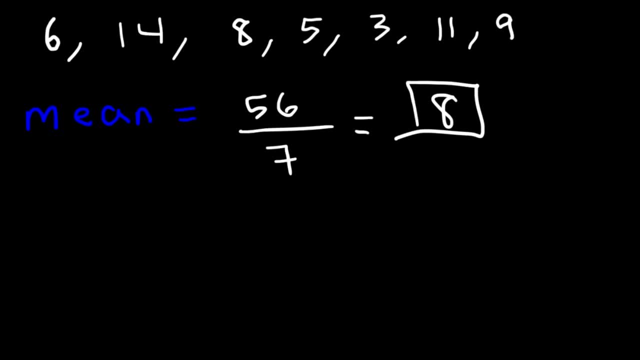 So the average or the arithmetic mean is equal to eight. So now let's go ahead and calculate. Okay, So let's find the median. But to do that let's arrange it and increase. in order: The lowest number is three. 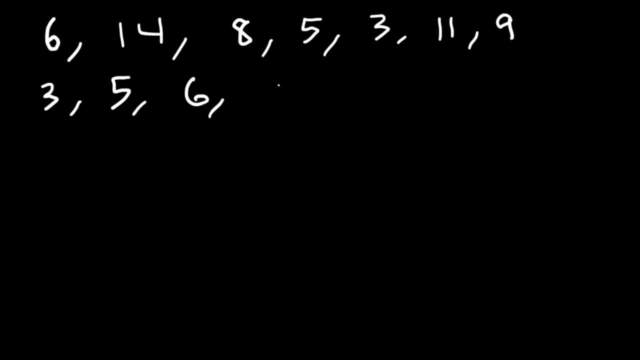 The next one is five, And then we have six, eight, nine, eleven and fourteen. Notice that the middle number is eight. So therefore, the median is equal to eight. Now, what about the mode? What is the value of the mode in this problem? 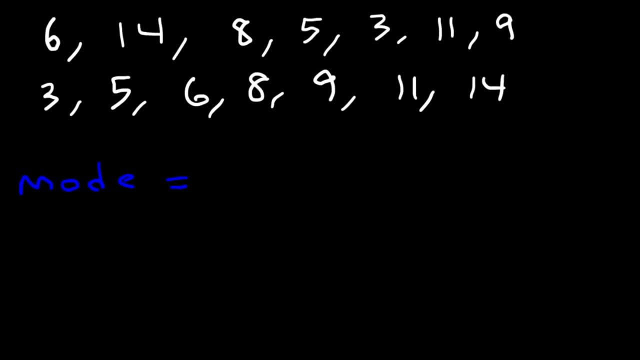 Which number occurs most frequently? Notice that every number occurs only once, So therefore there's none. There is no mode in this particular problem. Now, the last thing that we need to figure out is the range, which is the difference between the highest number and the lowest number, The 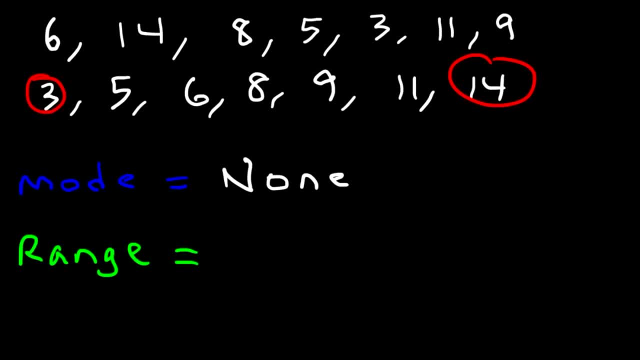 highest number is 14,, the lowest number is 3,, and so 14 minus 3 is equal to 11,, and so that's the range So far. we've considered two examples in which we had an odd number of numbers in a data set. In this case, there was only seven. 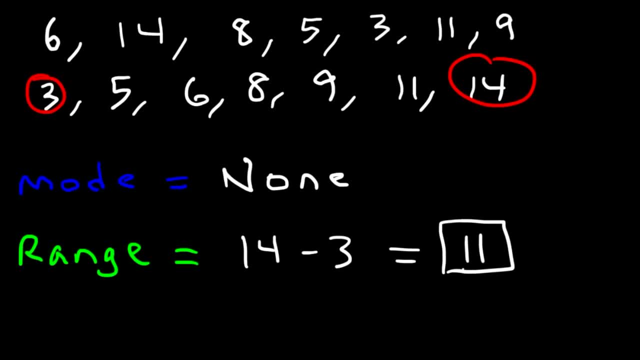 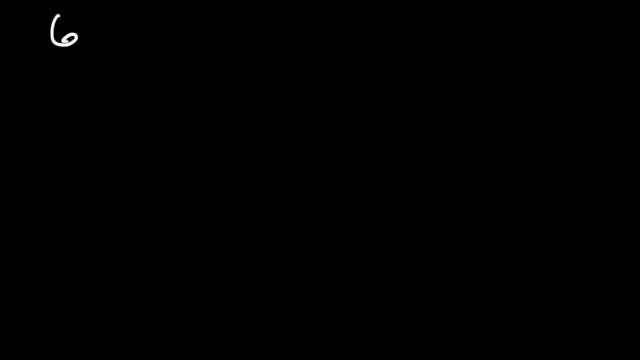 numbers. but what if we have an even number of numbers? For example, let's say, if there are eight numbers in a data set? Let's try this example. Let's say the numbers are 6, 8,, 5,, 5,, 9,, 8,, 10, and 8.. So go ahead, take a minute, calculate the. 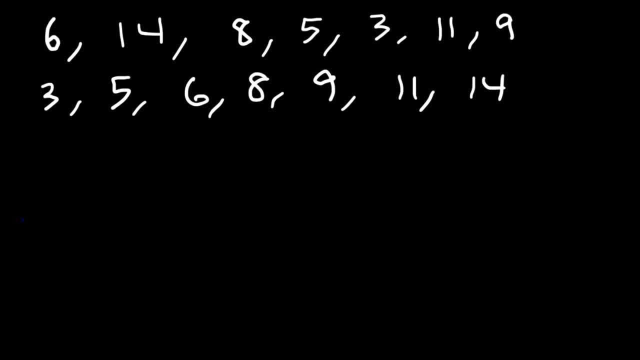 eight. now what about the mode? what is the value of the mode in this problem? which number occurs most frequently? notice that every number occurs only once, so therefore there's none. there is no mode in this particular problem. now, the last thing that we need to figure out is the range, which is the difference. 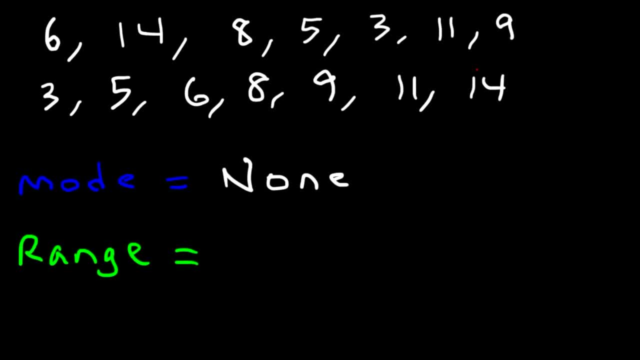 between the highest number and the lowest number. the highest number is fourteen, the lowest number is three, and so fourteen minus three is equal to eleven, and so that's the range so far. we've considered two examples in which we had an odd number of numbers in the data set in. 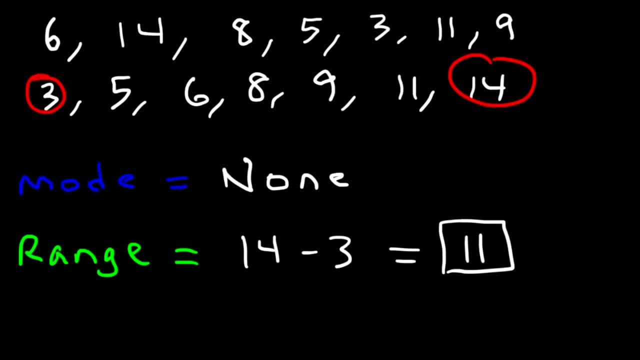 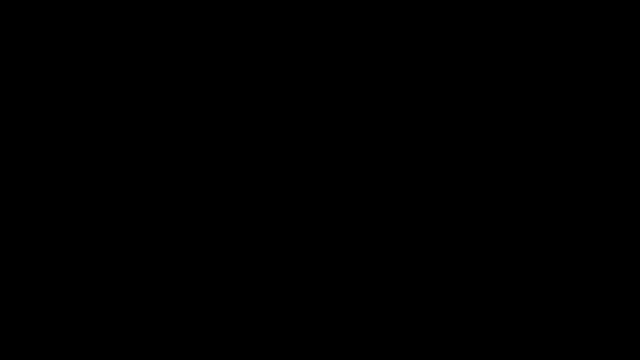 this case there was only seven numbers. but what if we have an even number of numbers? for example, let's see if there are eight numbers in a data set. let's try this example. Let's say the numbers are 6,, 8,, 5,, 5,, 9,, 8,, 10, and 8.. So go ahead, take a. 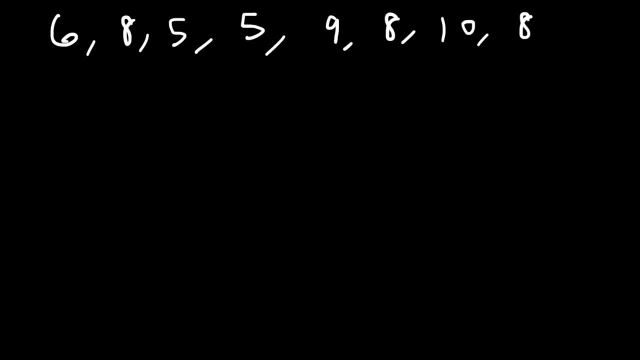 minute calculate the mean, median mode and range. So let's start with the mean. Let's add up the numbers: 6 plus 8 plus 5 plus 5 plus 9 plus 8 plus 10 plus 8 will give us a sum of 59, and there are eight numbers Now. 59 divided by 8 is: 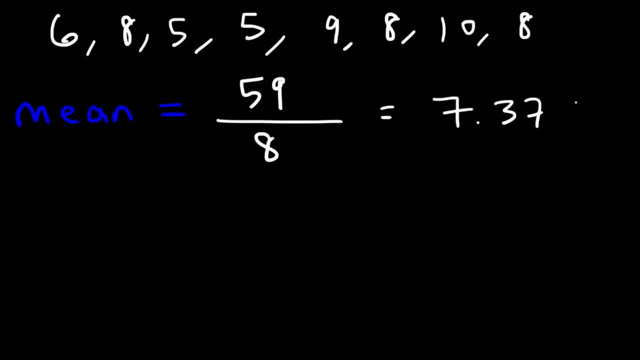 equal to 7.375, and so this is the average. Now let's calculate the mode. Now, before we do that, let's put the numbers in increasing order, as we did before. So the lowest number is 5, there's 2 of them, and then we have a 6, there's 3, 8's, there's. 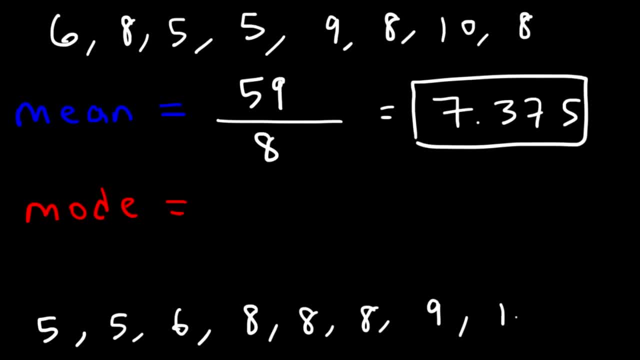 a 9, and there's a 10.. So notice that 8 is the number that occurs most frequently. there's 3 of them, So the mode is 8.. Now the median is going to be the middle number. Let's see, we can get rid of 5 and 10,, 5 and 9,, 6 and 6,, in this case the last 2 in the 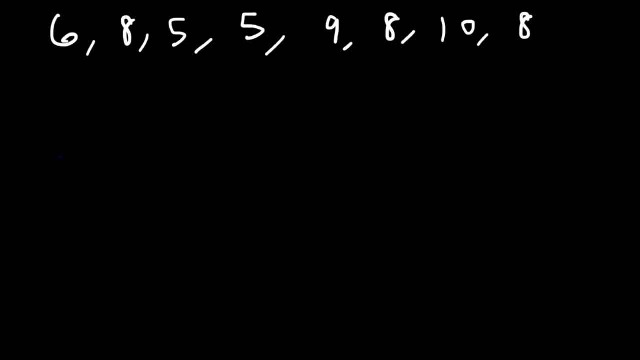 mean median mode and range. So let's start with the mean. Let's add up the numbers: 6 plus 8 plus 5 plus 5 plus 9 plus 8 plus 10 plus 8 will give us a sum of 59, and there are eight numbers Now. 59 divided by 8 is equal to. 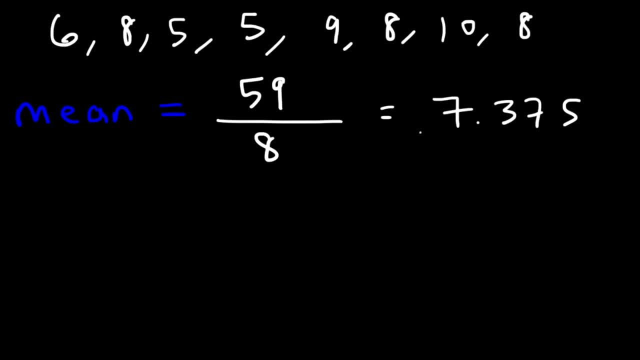 7.375, and so this is the average. Now let's calculate the mode. Now, before we do that, let's put the numbers in increasing order, as we did before. So the lowest number is 5, there's two of them, and then we have a 6, there's. 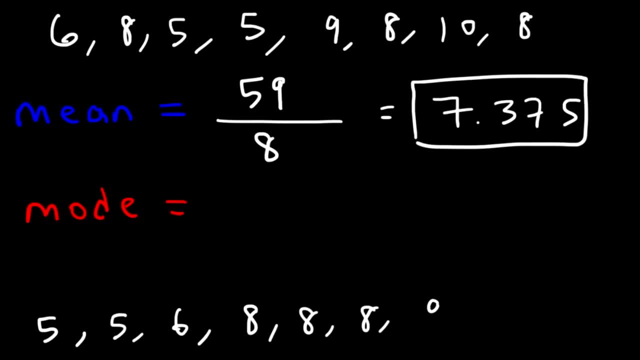 three 8s: there's a 9, and there is a 10.. So notice that 8 is the number that occurs most frequently. There's three of them, so the mode is 8.. Now the median is going to be the middle number. Let's see we can get rid of 5 and 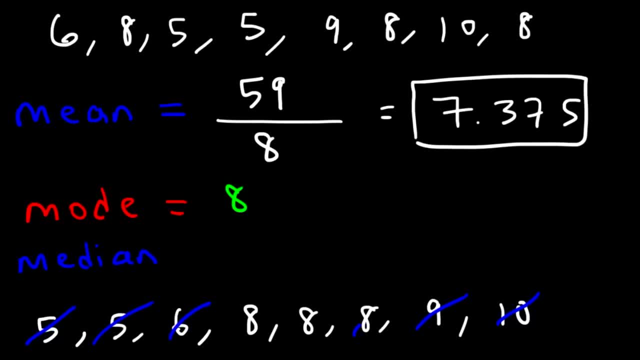 10, 5 and 9,, 6 and 6.. In this case, the last two in the middle are 8.. Because they're the same, the median is going to be 8.. Now, the last thing that we need to calculate. 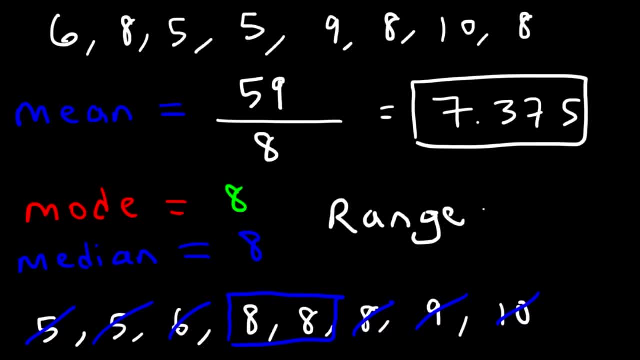 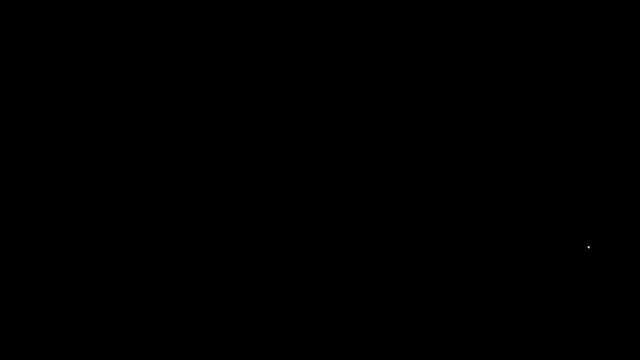 is the range, and we know the range is simply the difference between the highest number and the lowest number. So it's 10 minus 5, which is equal to 5.. Now let's work on one more example. This time we're going to have 10 numbers in a data. 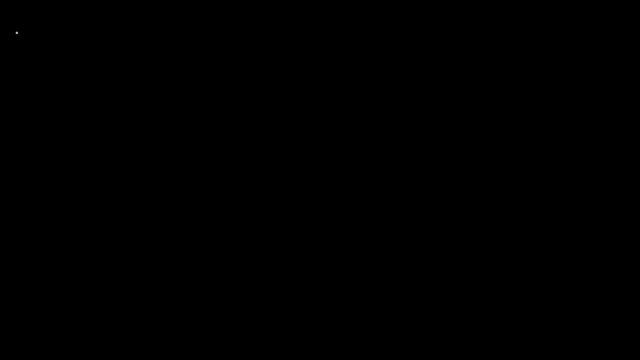 stat instead of 8.. So the numbers are 12,, 15,, 21,, 4,, 36, and 37. So we're going to have 15,, 11,, 48,, 29, and 38. So let's begin by calculating the mean. Let's add up the. 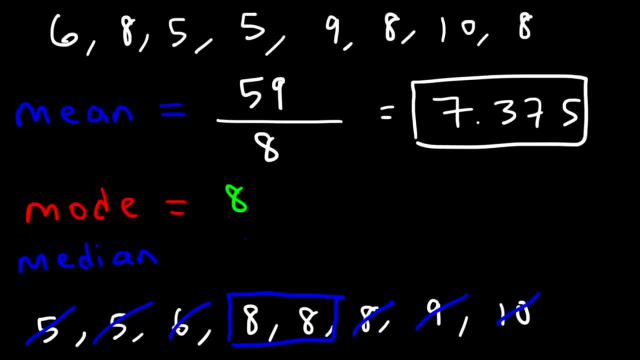 middle are 8.. Because they're the same, the median is going to be 8.. Now the last thing that we need to calculate is the range, and we know the range is simply the difference between the highest number and the lowest number. 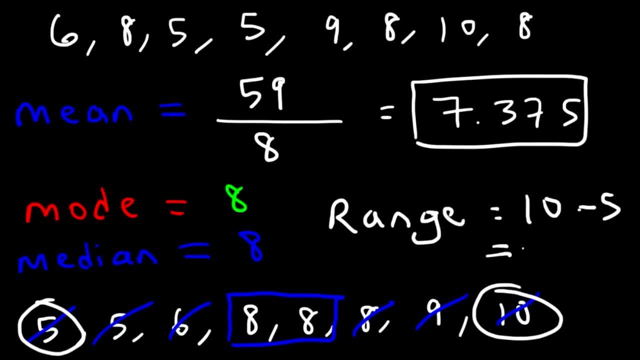 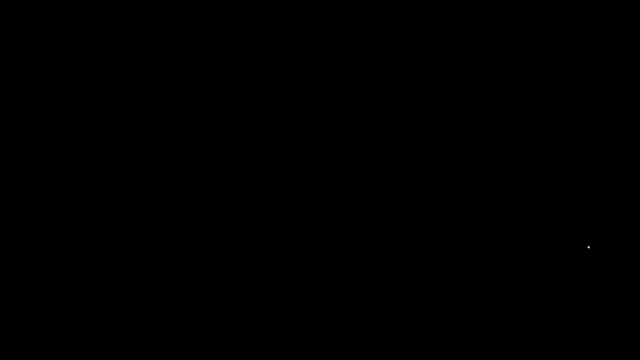 So it's 10 minus 5,, which is equal to 5.. Now let's work on one more example. This time we're going to have 10 numbers in a data set instead of 8. So the numbers are 12,, 15,, 21,, 4,, 7, 8.. 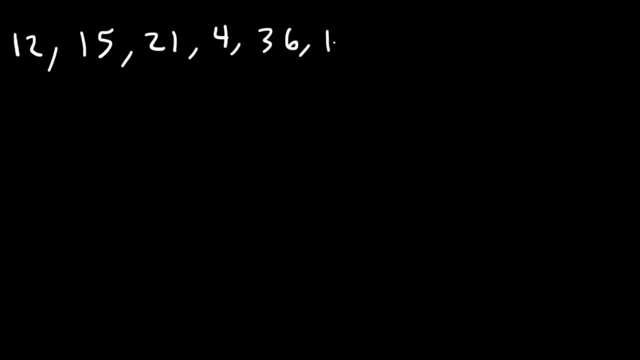 36,, 15,, 11,, 48,, 29, and 38.. So let's begin by calculating the mean. Let's add up the 10 numbers, So the sum of the 10 numbers is 229.. 229 divided by 10 will give us an average of 22.9.. 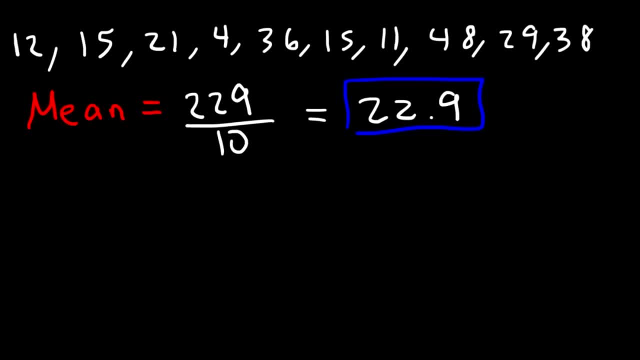 So that's the arithmetic mean. Now let's calculate the median. So let's put everything in order. The lowest number is 4, and then we have 11, and then 12,. there's two 15s, next we have 21,, 29,, 36,, and then 38 and 48.. 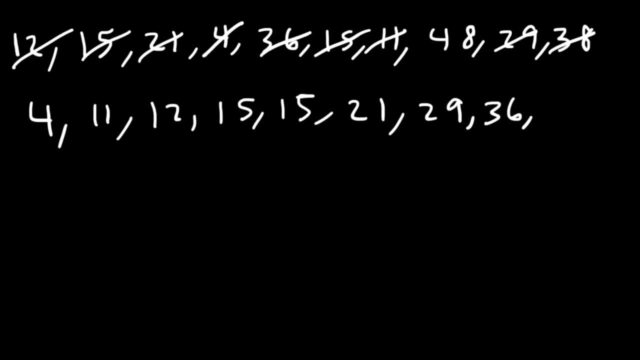 So that's the median. Now let's calculate the mode. 15 is the number that appears most frequently, So the mode is going to be 15.. Now to find the median, we need to calculate the middle number. What do you think the middle number is going to be?